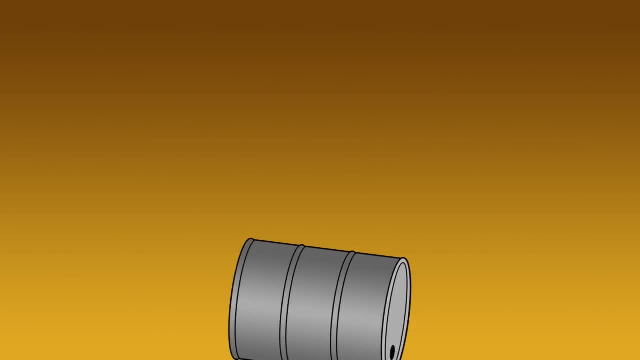 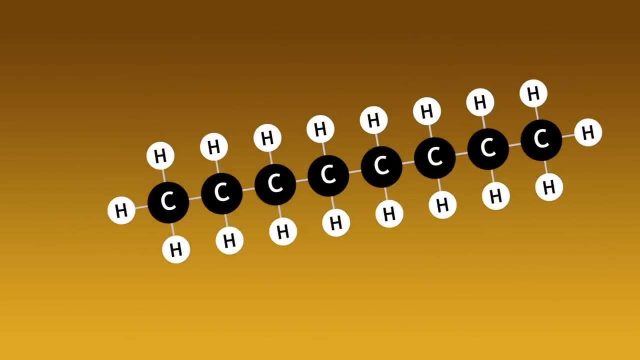 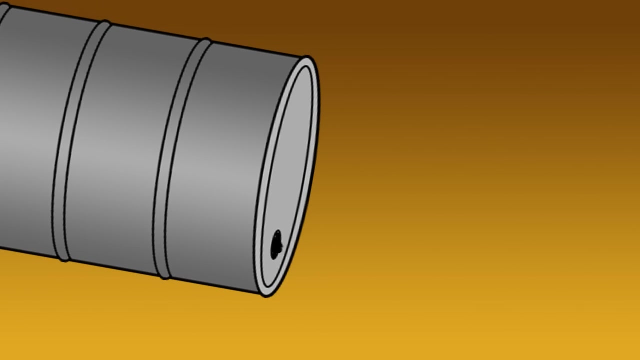 valuable resource. It provides us with a great number of hydrocarbons, some of which are useful as fuels and others are used in the manufacture of many different chemicals and even plastics. However, in the raw form, as crude oil, it can be a viscous, dark coloured. 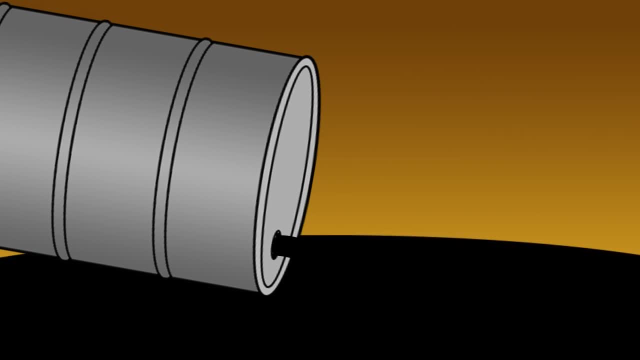 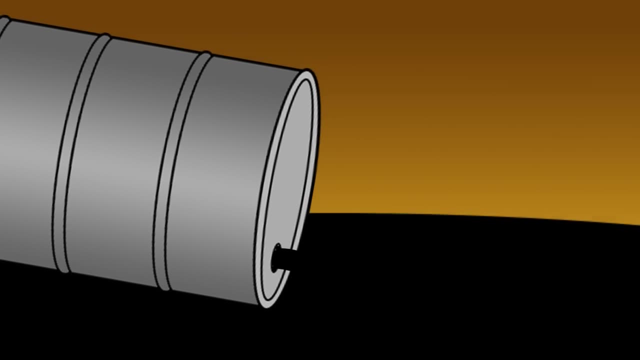 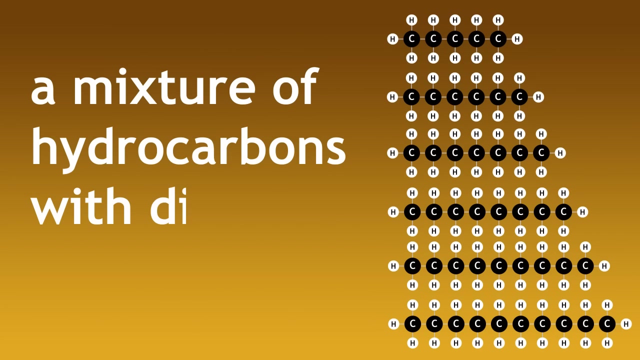 tar-like consistency and the different fractions of hydrocarbons must be separated by fractional distillation for them to be useful. Before we understand how fractional distillation works, we should be clear that crude oil is a mixture of hydrocarbons with different chain lengths, some being short molecules and some 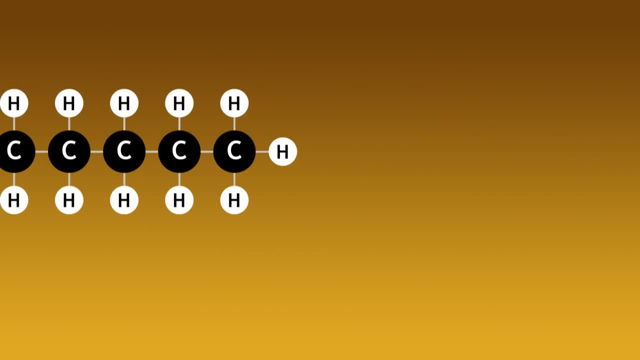 being very long. Intermolecular forces act between molecules, and the longer the molecule, the greater the intermolecular force. As you can see here, the small molecules have weaker intermolecular forces and so will require less energy to be produced. 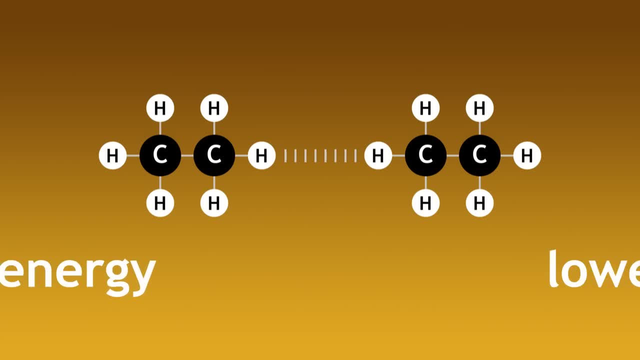 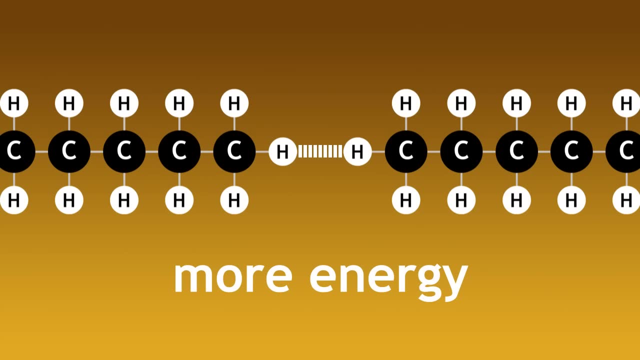 To break them apart and turn them into a gas. they have a lower boiling point. The longer molecules have greater intermolecular forces. More energy is required. A higher temperature will be needed to evaporate these molecules. They have a higher boiling point. 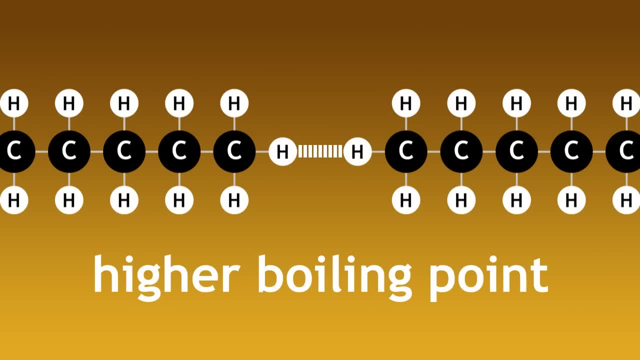 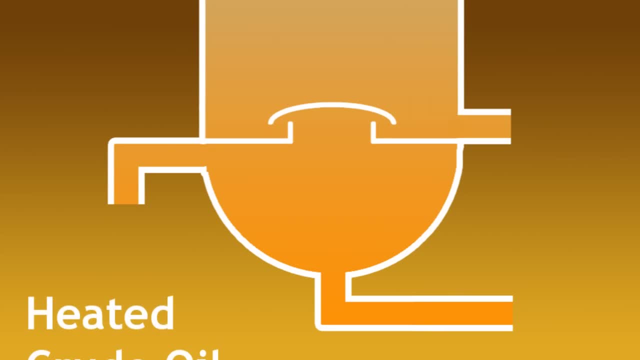 Now we understand how chain length is related to the boiling point of a molecule. let us look at how this method works. As you can see, crude oil is heated up to a temperature of about 20 degrees Celsius, and it is heated up to a temperature of about 20 degrees Celsius. This is the temperature. 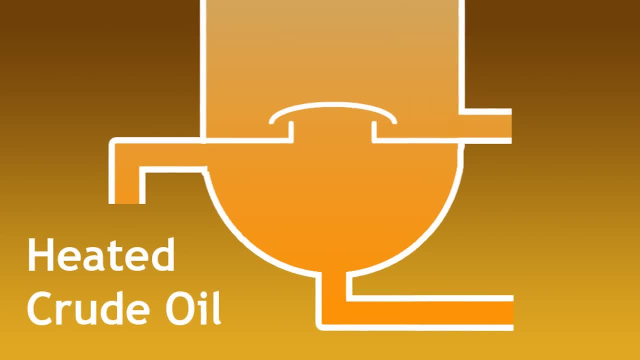 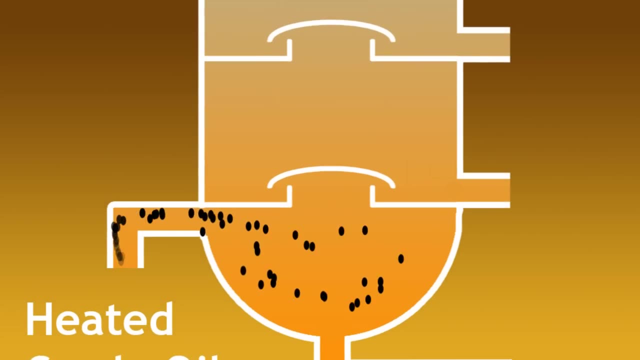 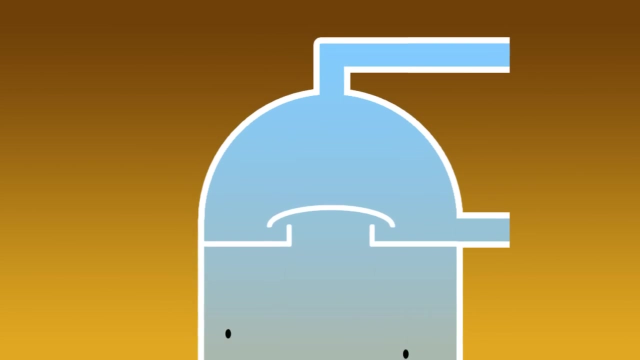 that is heated up to a high temperature outside of the fractionating column, The hot crude oil, now mostly in vapour form, is pumped into the column. The column has a heat gradient and is very hot at the bottom, going cooler as we move up to the top, Even at the very 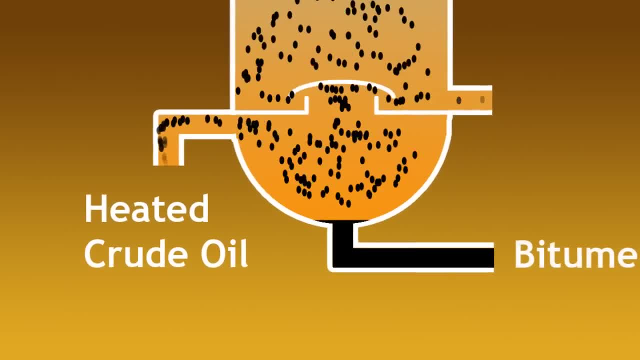 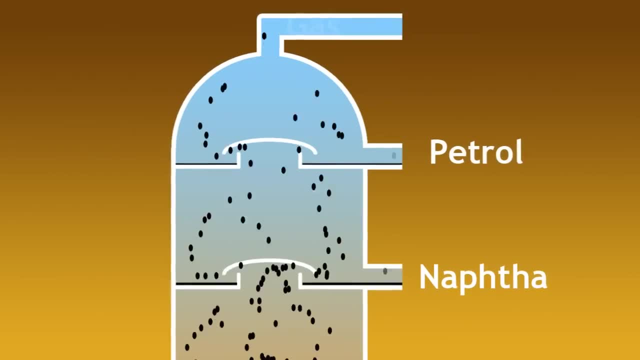 bottom of the column, where the temperature is still high. some long chain molecules with high boiling points begin to condense back into a liquid. These are collected at the bottom of the column. The rest of the molecules start to rise up the column, making their